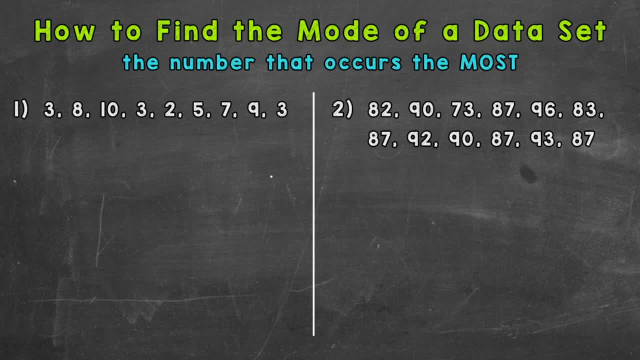 So we're going to go through two examples here and find the mode in order to help you get this down. So let's jump right into number one here, And the first thing we need to do is take our data set and put it in order from least to greatest. 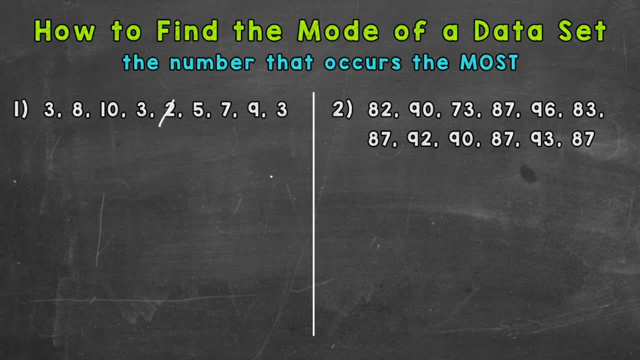 So our smallest number in value is this two here. So I cross it off That way. I know I counted it And I don't skip anything or count anything twice. So after that it looks like we have three, threes. So one, two, three. Then we have a five, a seven, an eight. 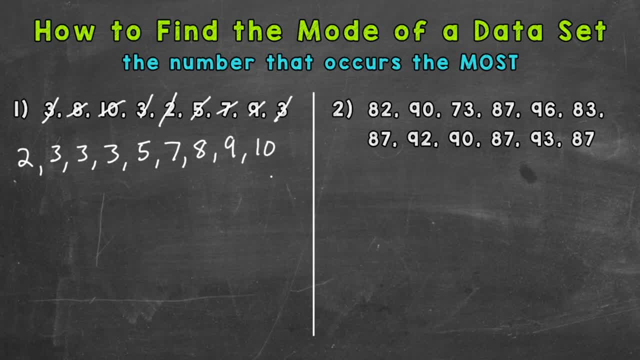 a nine and lastly a ten. So just to just to double check, let's see how many numbers we had in our data set: One, two, three, four, five, six, seven, eight, nine- And then we double check that with our list. 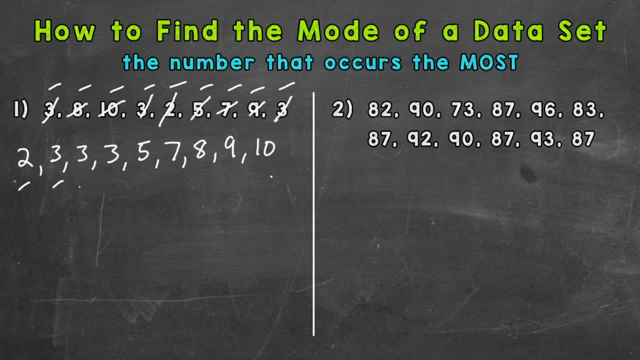 to make sure they match One, two, three, four, five, six, seven, eight, nine. So we are good, good to go. So our mode is going to be our three. here We have three, threes, So that occurs the most. 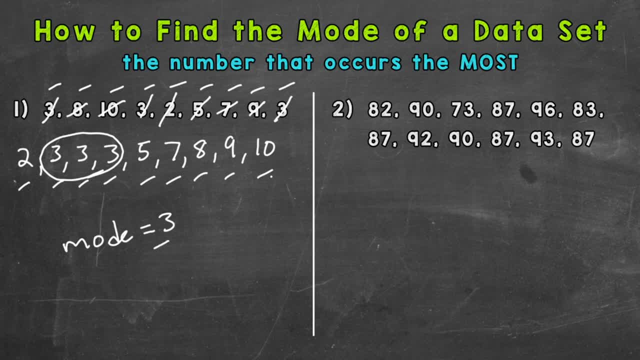 So mode equals three. So it's as simple as that for mode. whatever occurs the most, So number two. let's put them in order from least to greatest. So our smallest number in value is going to be this: 73.. Then we have it looks like an 82.. 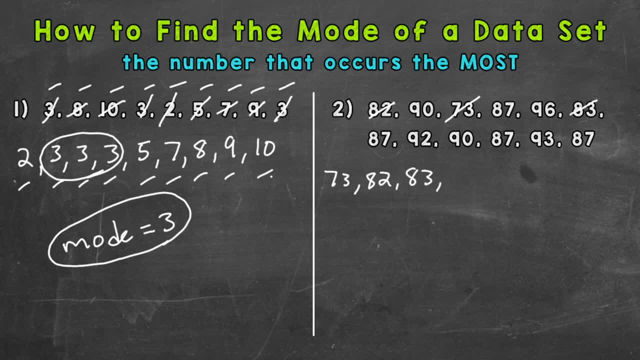 Then an 83.. And it looks like four 87s come. next One, Two, Three, Four, Then we have a 90.. I'll go to the next line down here. Uh, two 90s, A 92.. 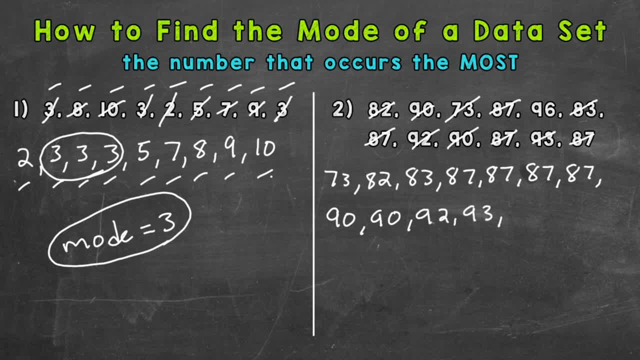 And a 93. And lastly a 96.. So let's double check here: One, two, three, four, five, six, seven, eight, nine, 10.. eight, nine, 10,, 11,, 12,. one, two, three, four, five, six, seven, eight, nine, 10,, 11,, 12.. So